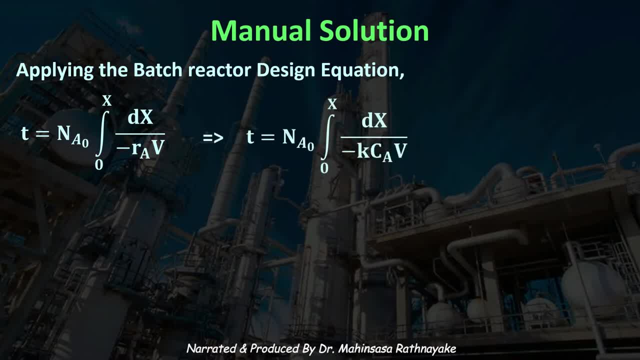 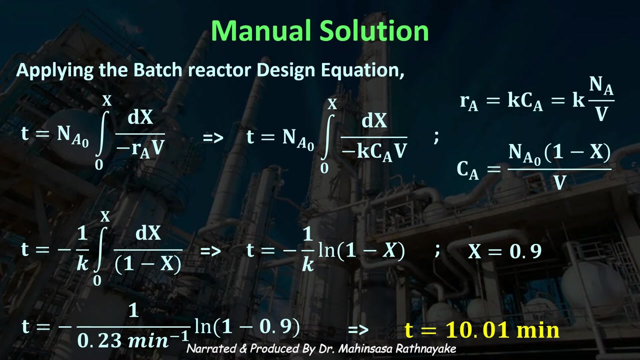 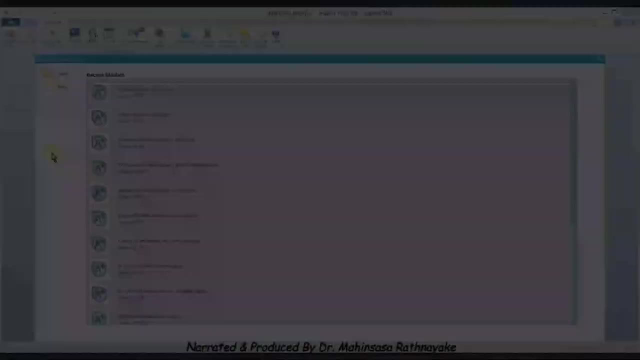 You can see the solution on the screen now. The result is as follows. The manual calculation result gives an answer as 10.01 minutes to reach 90% conversion. Now let's see the simulation procedure and simulation result for this problem in Aspen Plus software. 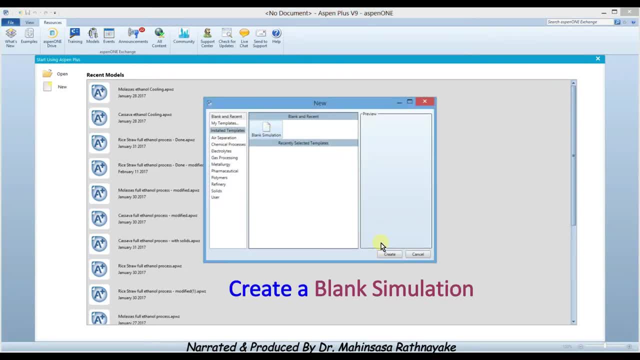 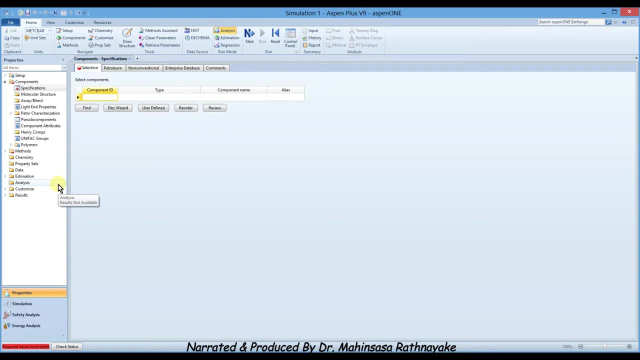 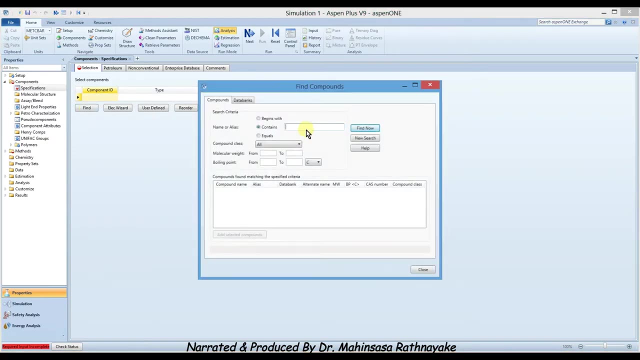 Create a new simulation in Aspen Plus using the blank simulation option. Specify cis-2-butene as 0.25.. The result is as follows. The result is as follows: Specify cis-2-butene and trans-2-butene under the components. 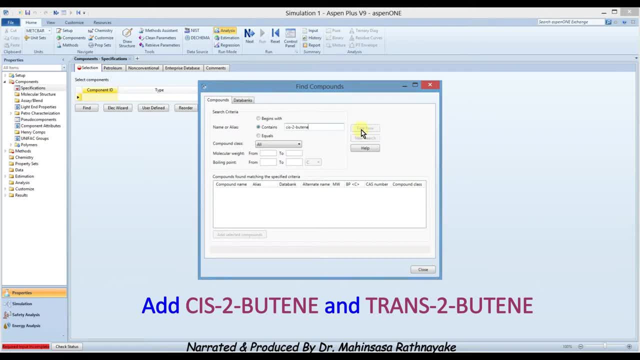 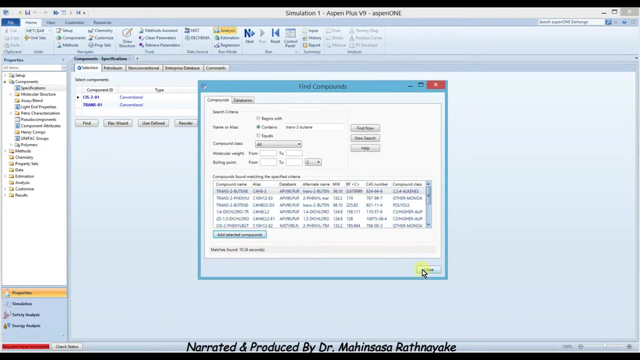 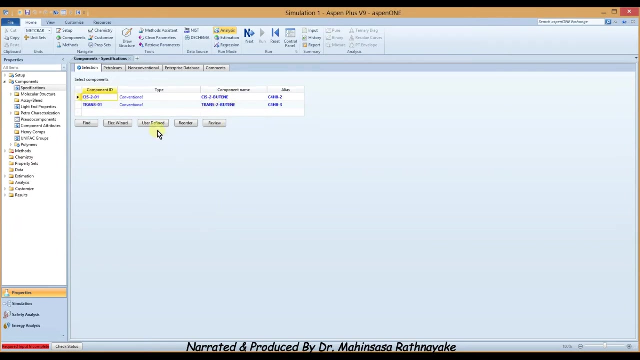 The result is as follows. The result is as follows: Rename the component IDs as cis and trans respectively. A warning message will appear saying that the component ID to be renamed. Click Yes. No changes happen to the component properties, except the component ID. 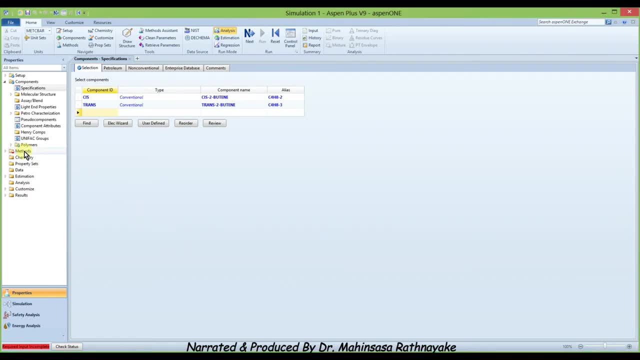 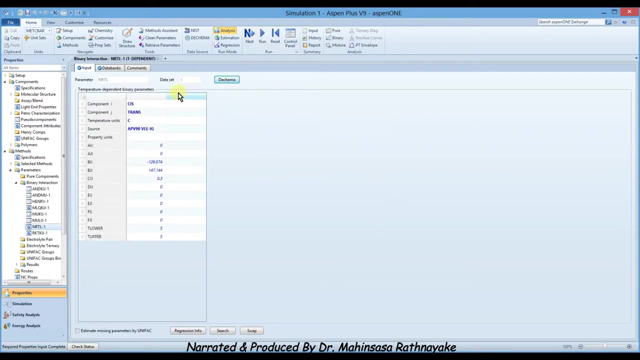 Go to Methods Specifications- global sheet. Set the base method field to Non-random-to-liquid property method, which is abbreviated as nrtl. click the next button to populate the binary interaction parameters. move to the simulation environment by clicking the simulation button at the bottom left of the screen. 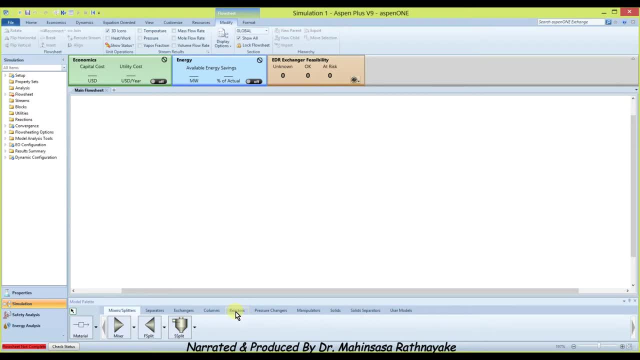 go to the reactors tab of the model library and select our batch block and drop it to the main flow sheet. connect two material streams for batch charge or feed and reactor product. rename the streams and the reactor block properly by pressing ctrl plus M or right-clicking. 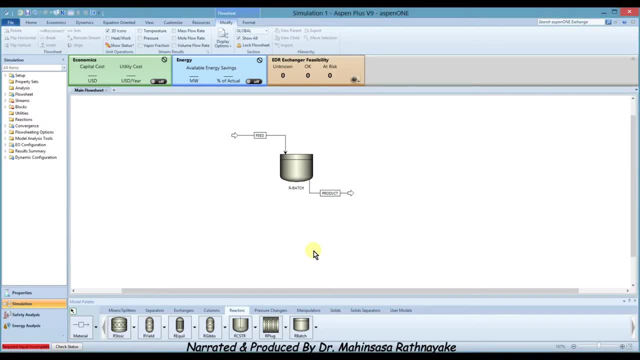 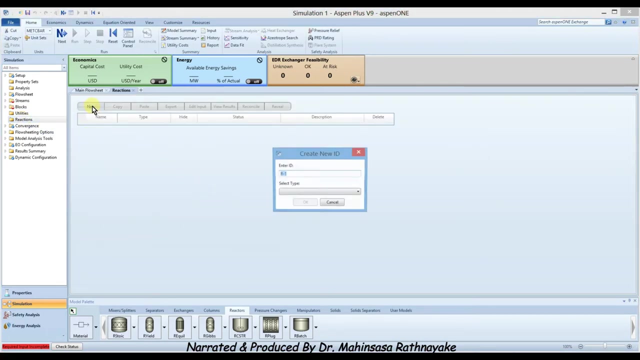 note that the our patch block can model a specified reaction using the kinetic data and specified residence time. however, it is still a steady-state model in the navigation pane. go to reactions. new select general for reaction type. by default, reaction ID r1 will be created or you can create a new ID. 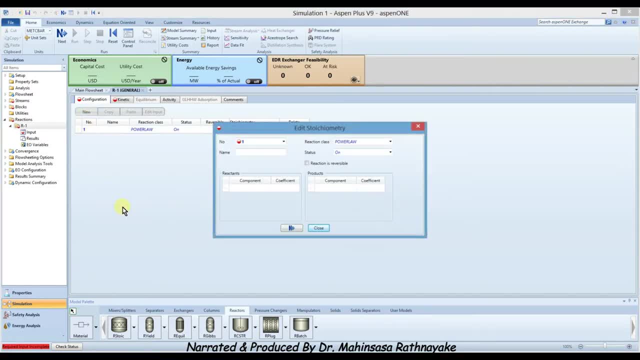 as you wish. go to reactions r1 and click new. enter reaction 1 as the reaction name. so we type rxn1 in short form. select cis 2 butene for the reactant component and trans 2 butene for the product component, as well the stoichiometric coefficients. 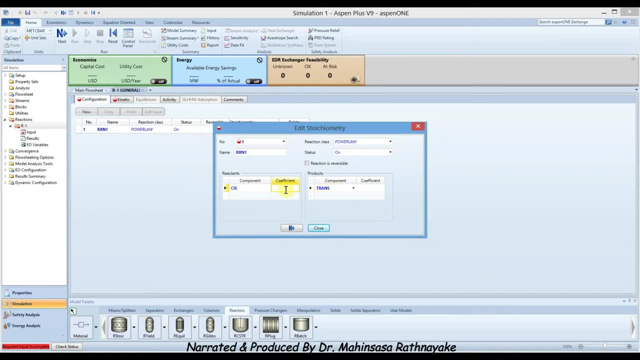 in the balance reaction should be 1 for both cis 2 butene and trans 2 butene. notice that the coefficient for the reactants automatically becomes negative. to mark the material balance, click close. after completing the reaction. then define the reaction kinetics in reaction group r1. go to the kinetic tab. 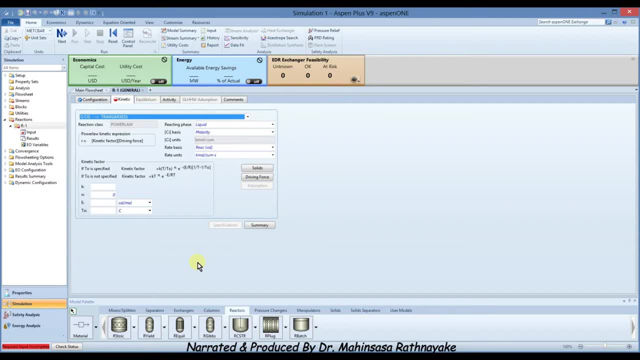 enter simple k is equal to 0.003833. note that the default units for rate constant should be per second. then enter activation energy. capital E is equal to zero. we can see that simple k in aspen plus refers to pre-exponential factor. when activation energy is 0, the pre-exponential factor equals to the rate constant simple. 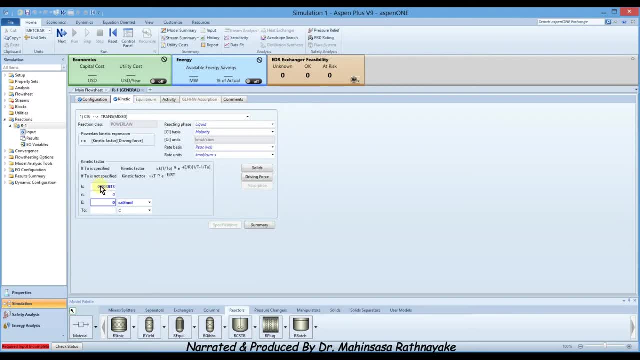 k according to Arrhenius equation. keeping the mouse cursor over an input field will show the text giving information about it. clicking into the field and pressing f1 brings up the aspen plus help page on the topic. let's do this in the field for k in aspen plus calculation. 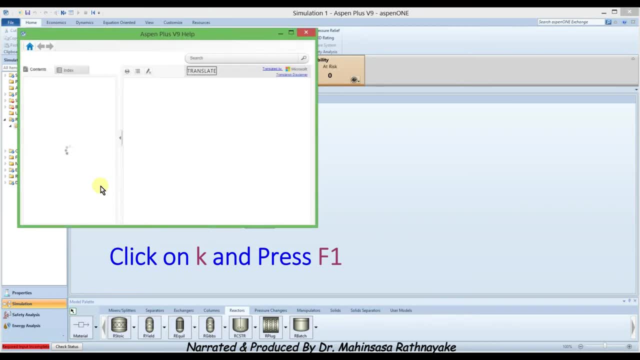 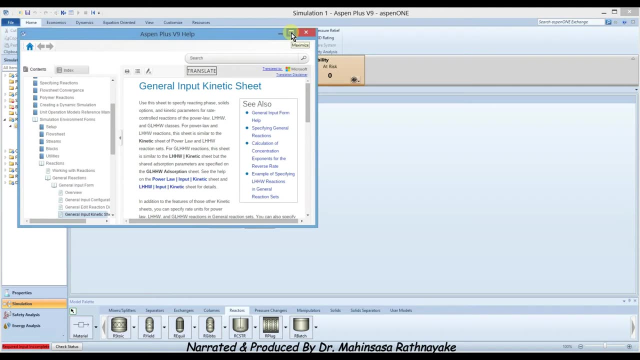 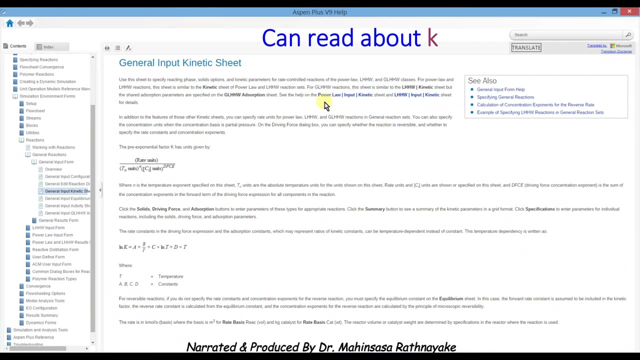 open the Aspen plus help page and this is what we get. we get a new reaction by setting Click OK to see the help page about the pre-exponential factor and the respective equation. Next, select the driving force button. Enter 1 as the component for cis2 butene. 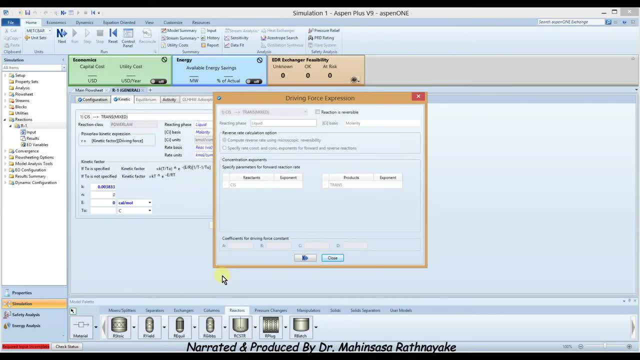 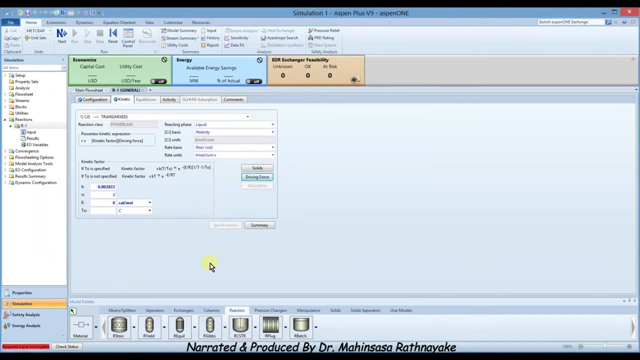 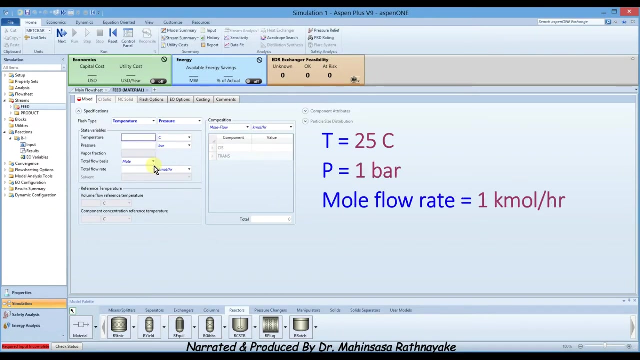 And specifies the reaction order in the kinetic rate law. After completing the input entries, close the window In the navigation pane. go to Streams- Feed Input. Enter 25 degree Celsius for temperature, One bar for pressure And a mol flow of 1 kilomol per hour for component cis2-butene. 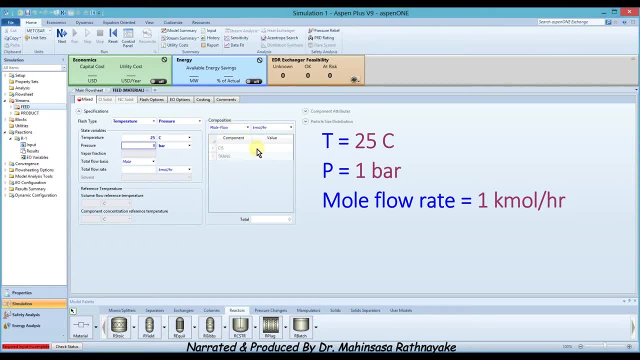 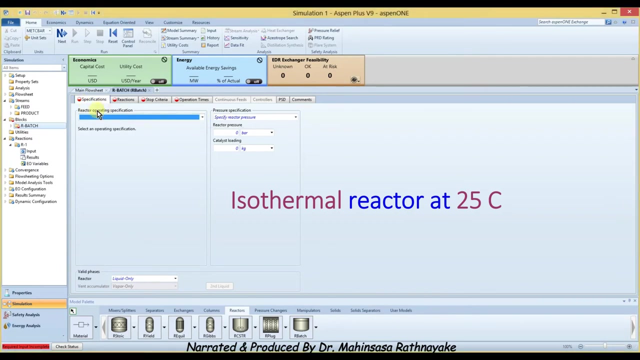 Note that if you enter individual component flow into the composition section, it is not required to enter the total flow. Go to Blocks R-Batch Setup. In the Specification field, select Constant Temperature and enter a temperature of 25 degree Celsius. Note that this is not a realistic reactor temperature. 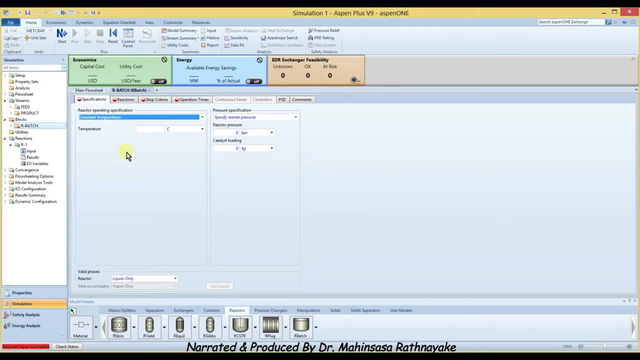 However, our kinetics are not temperature dependent and it is acceptable for this simplified example. Next, enter the reactor- operating pressure. You may enter the operating pressure by entering a pressure greater than zero, or you can specify the pressure drop through the reactor by entering a number less than or equal to zero. 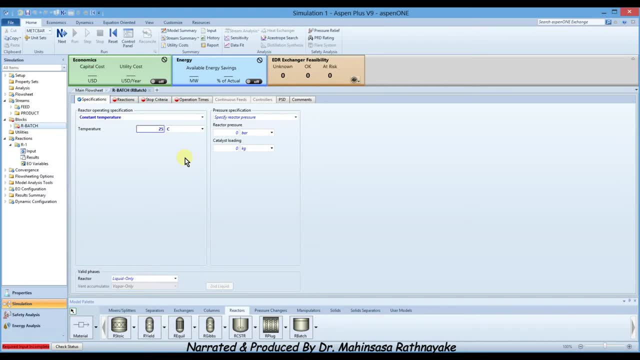 In this case, enter zero for reactor pressure, which means that this reactor will not experience any pressure drop and will operate at the given feed pressure of one bar. In the Reactions tab, specify R1 as the selected reaction sector. Specify stop criteria in order to stop computation when the conversion reaches a designated value. 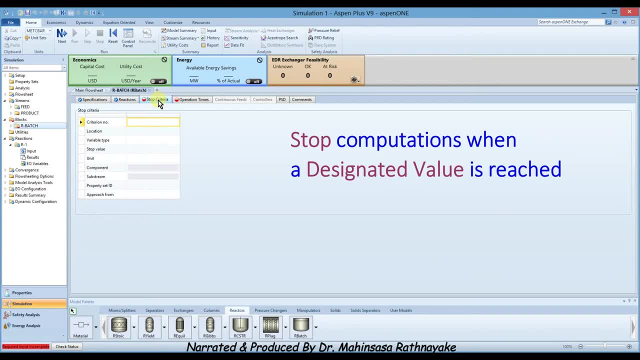 In this case, when the mole fraction of trans-2-butene in the reactor reaches 0.9,. that means 90% conversion. reactor computations should be stopped. The product stream will have the composition of the reactor at this designated value. 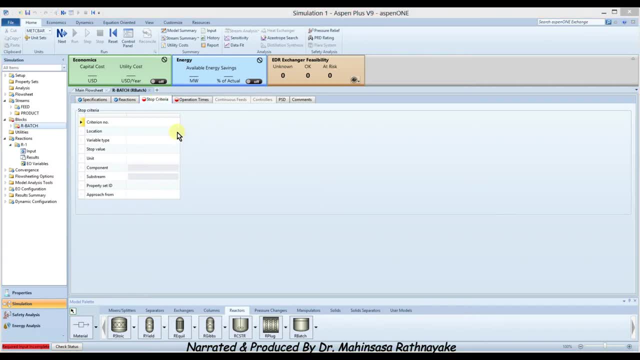 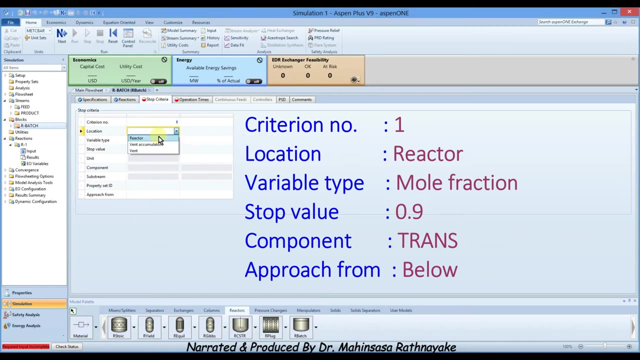 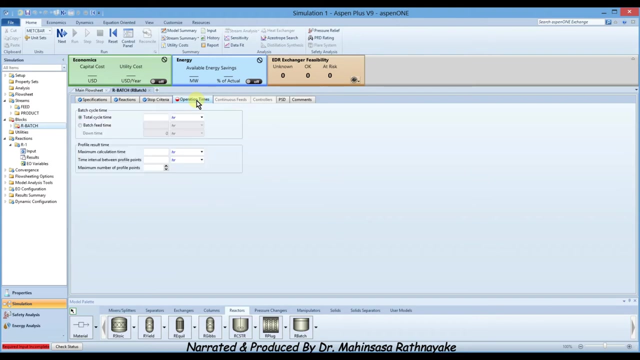 In the Stop Criteria tab. complete the input fields accordingly. Define operation time in order to create result tables and plots. Complete the input fields in the Operation Time tab. Total cycle time and maximum calculation time as 1 hour. total operation time and maximum calculation time as 1 hour. 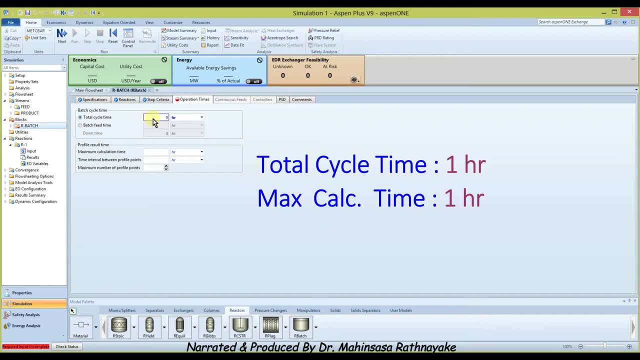 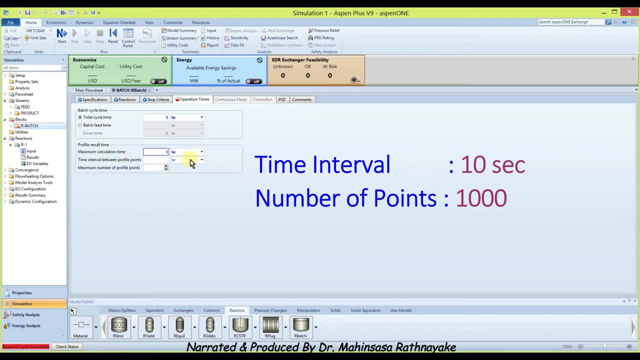 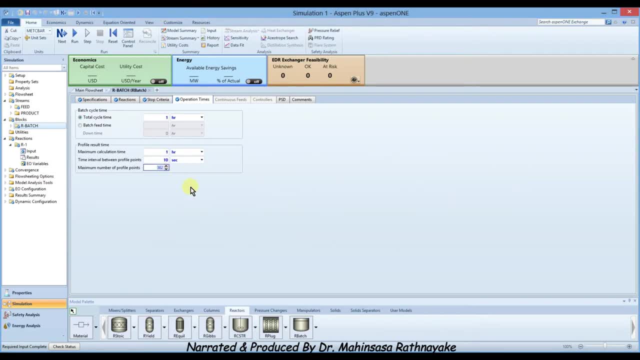 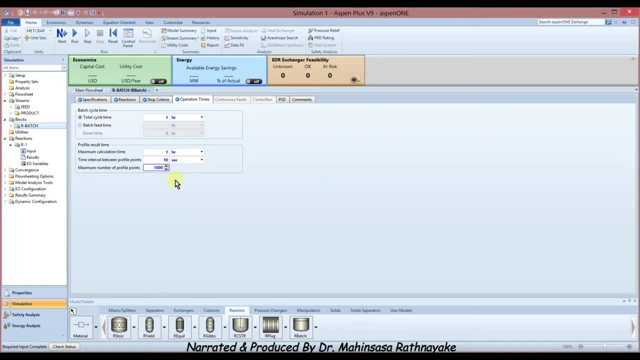 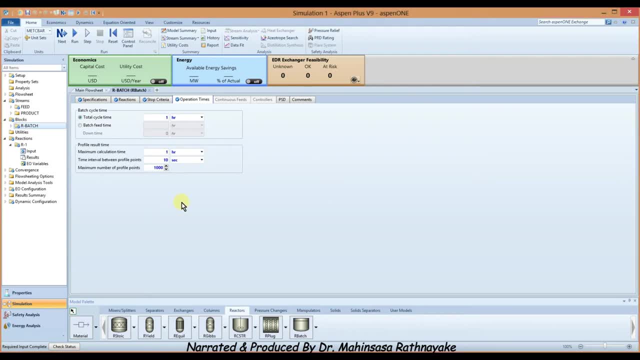 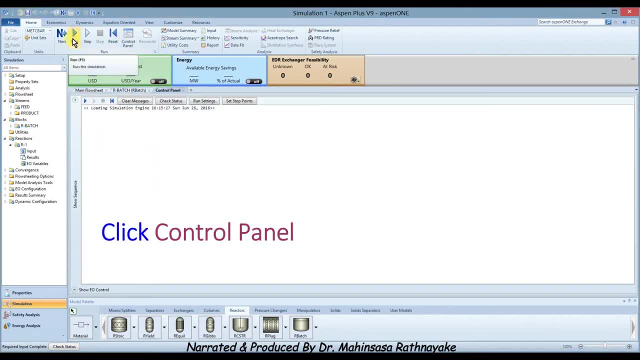 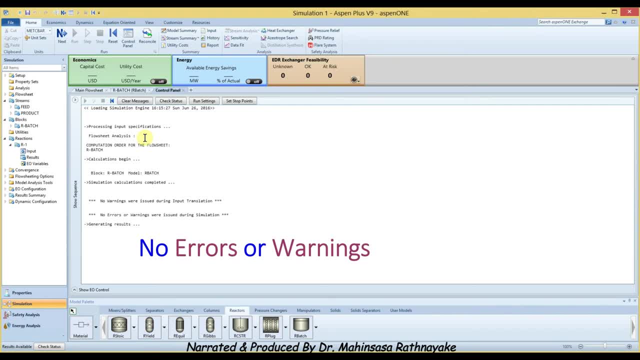 the user has to run the simulation always, While in Aspen HiSys software the user doesn't need to run separately, as the software automatically runs the simulation. After running the simulation, it shows that results are available. Go to the block's R-Batch Profiles Compositions tab. 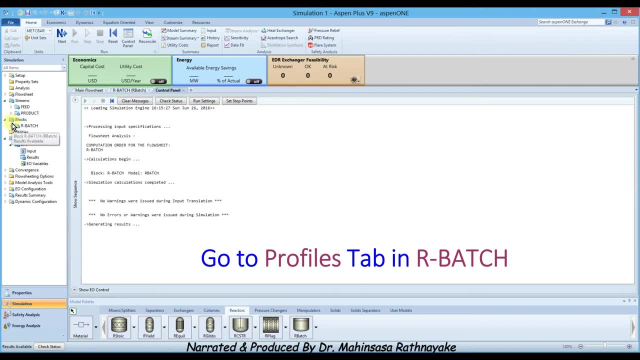 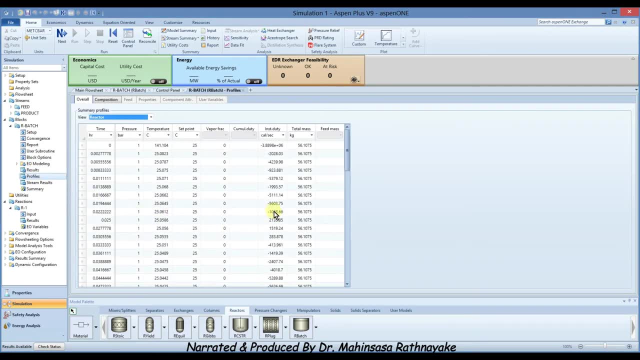 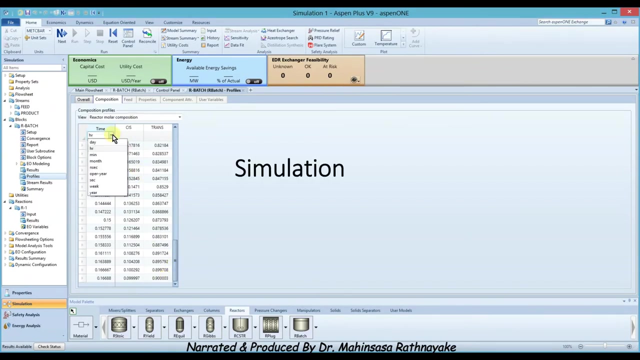 Go to the block's R-Batch Profiles- Compositions tab. The computed time is the number of times at which the trans-2-buty-mol fraction is 0.9 is shown as 10.01 minutes, which is identical to the manual calculation. 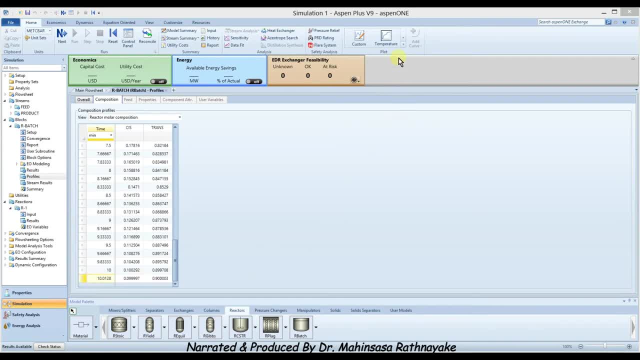 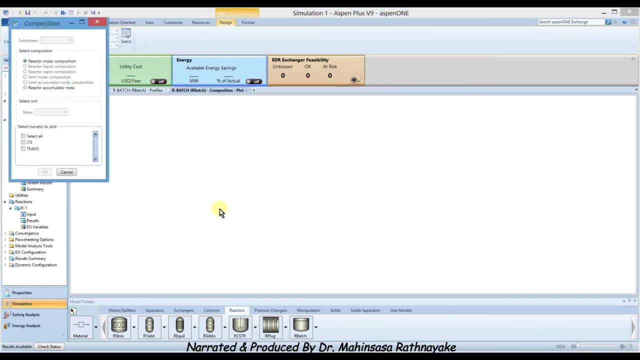 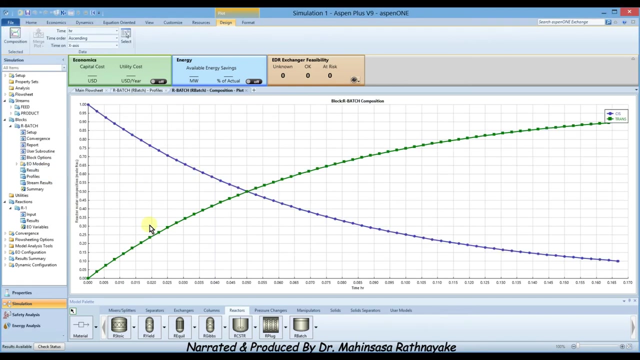 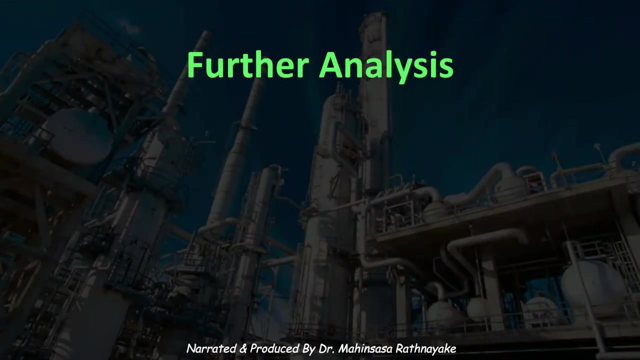 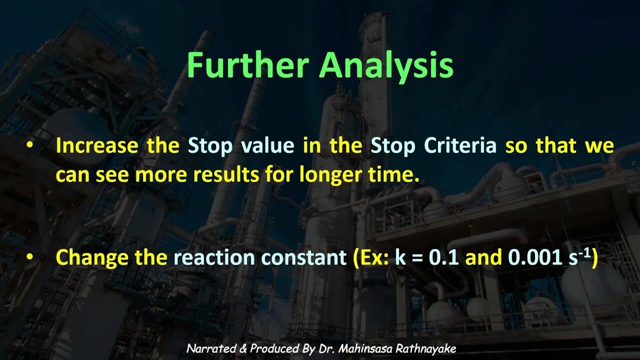 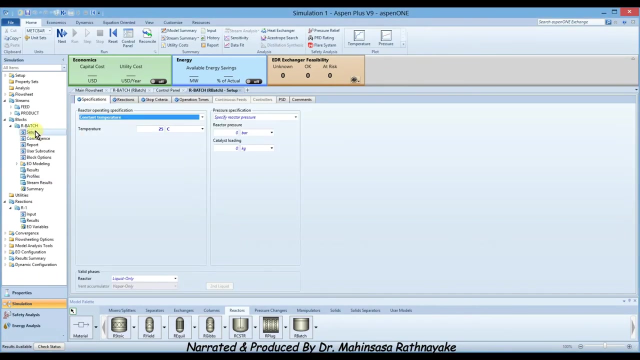 To see the composition variation: select Composition Plot in the ribbon. Select Composition Plot in the ribbon. Select Composition Plot in the ribbon. Use the For further analysis. we can perform following two variations. we can perform following two variations. Go back to the simulation and first increase the stop value in the stop criteria so that 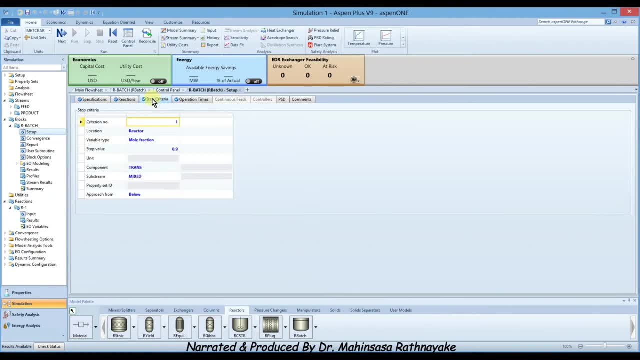 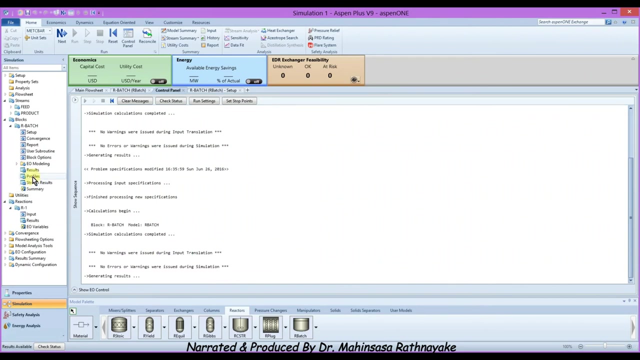 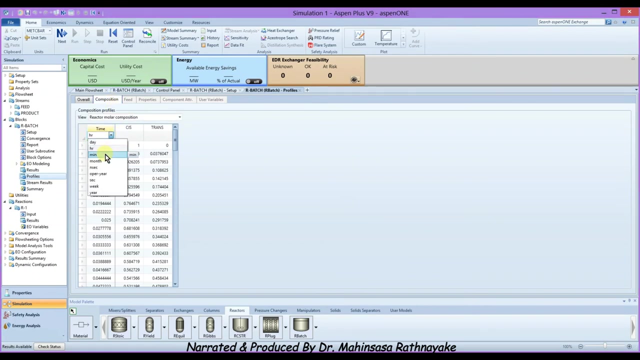 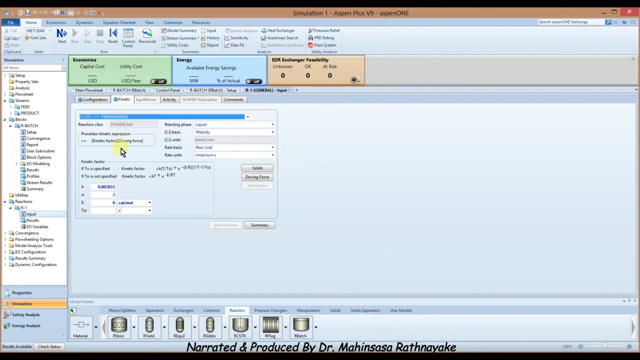 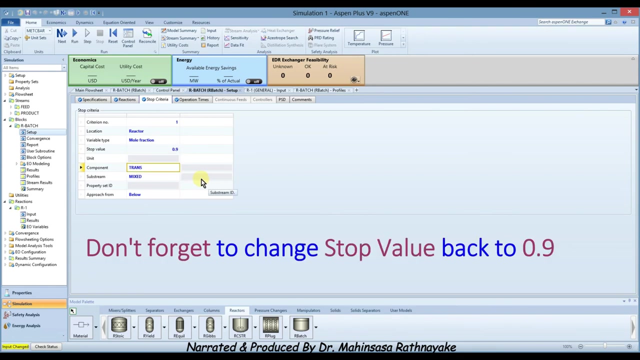 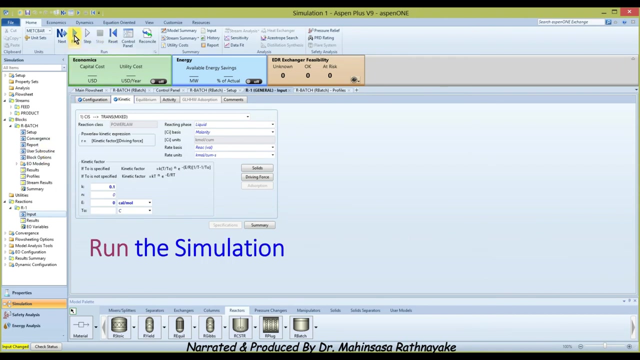 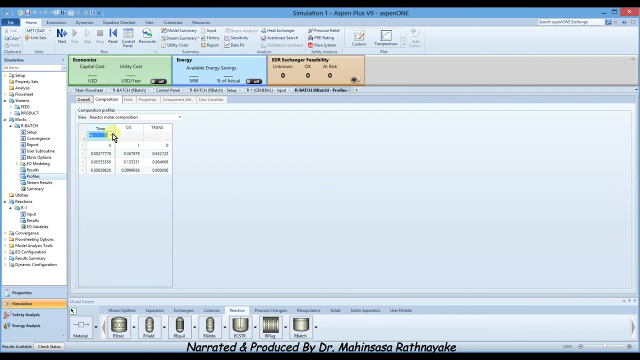 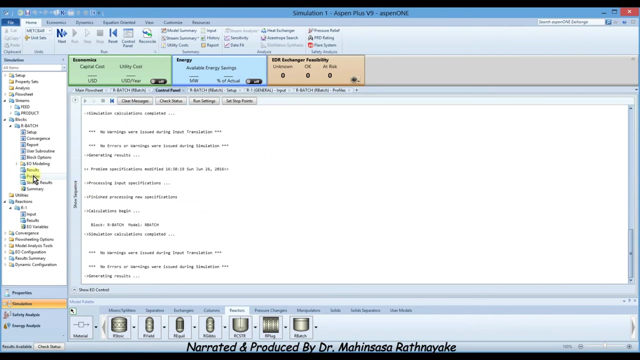 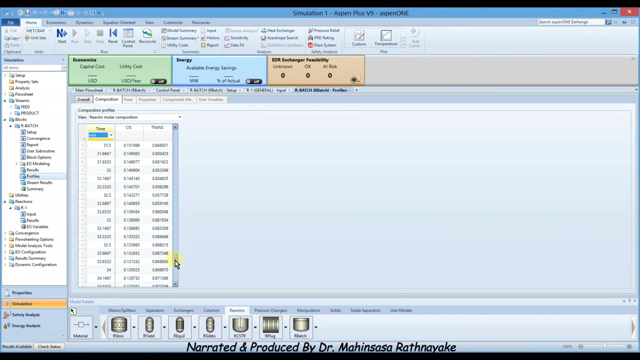 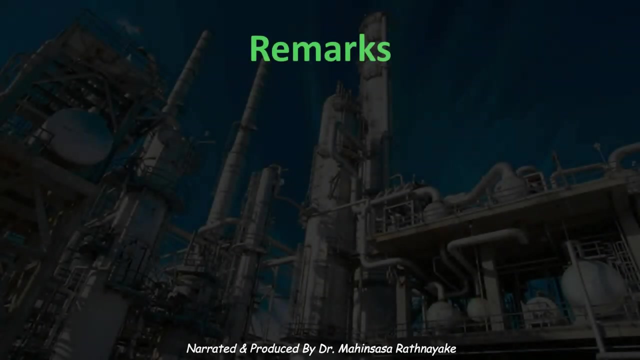 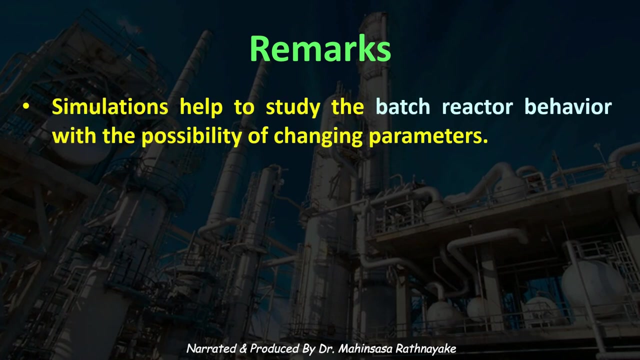 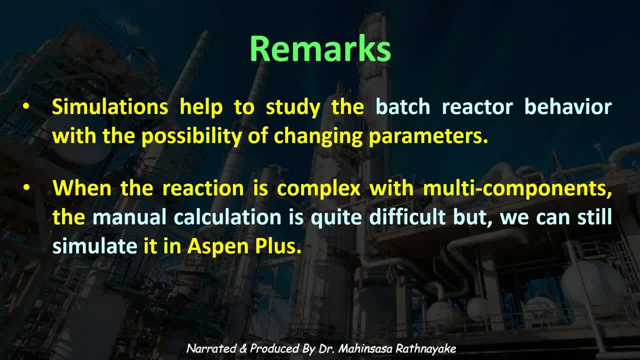 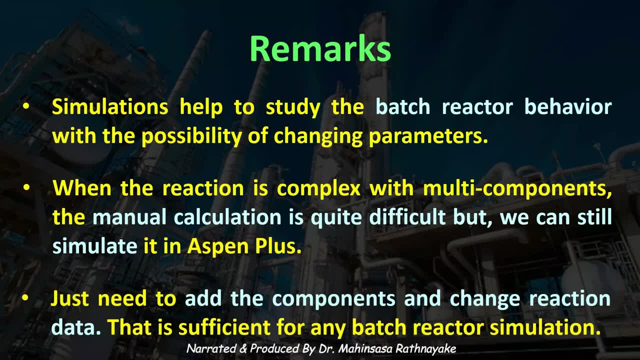 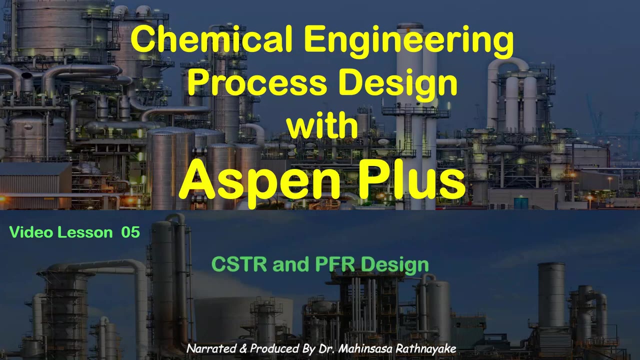 is quite difficult, but we can still simulate in Aspen Plus software. You just need to add the components and change the reaction data. That is sufficient for any batch reactor simulation. Please watch our next video lesson about CSTR and PFR design simulations using Aspen Plus.